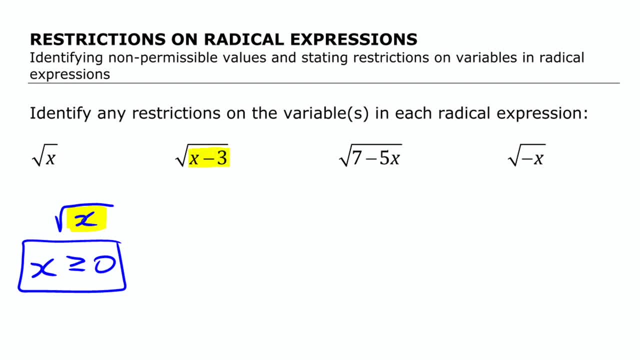 This one says square root of x minus 3.. This thing underneath here needs to be greater than or equal to 0. And the values of the variable that make that happen. if you're going to subtract 3 from them, well now, x doesn't have to be greater than or equal to 0,. 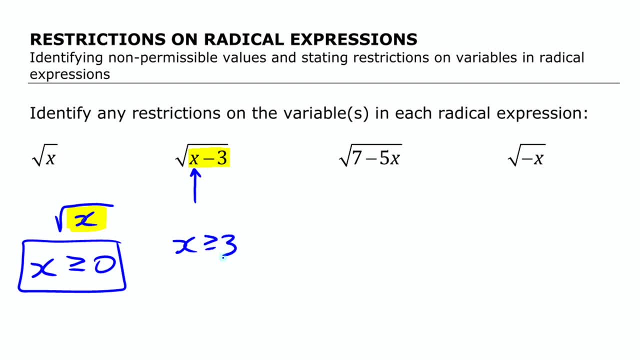 x has to be greater than or equal to 3.. If you put in numbers that are greater than or equal to 3 in there, like if you put 3, this is going to be 0. If you put 4, 4 minus 3, you get 1.. 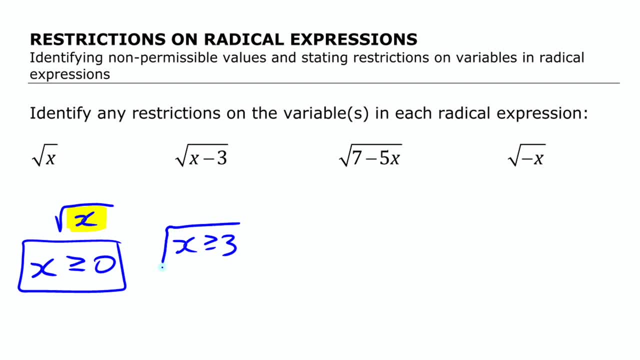 If you put any number bigger, it's going to be a positive number. That's the restriction on that expression, on that variable. For this one, maybe it's harder to see what the value of that variable is. So what we're going to do is we're going to just write an inequality. 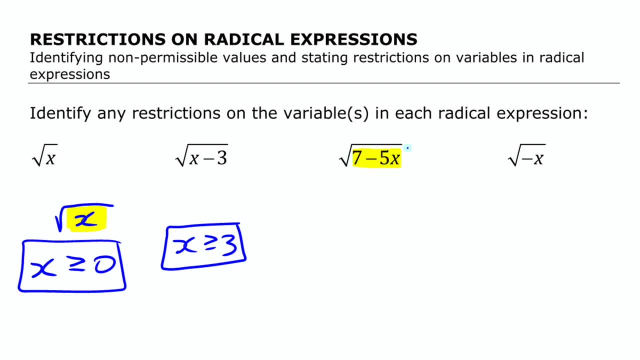 that says that that thing underneath the radical sign 7 minus 5x has to be greater than or equal to 0. If you can't see what it is right away, you can write an inequality like that and solve that inequality. 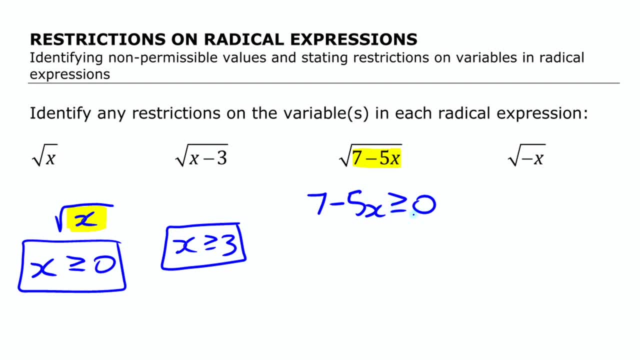 This says that 7 minus 5x has to be greater than or equal to 0.. I'm going to solve this inequality by moving that to the other side and making it positive 5x. I'm going to keep the sign the same way. 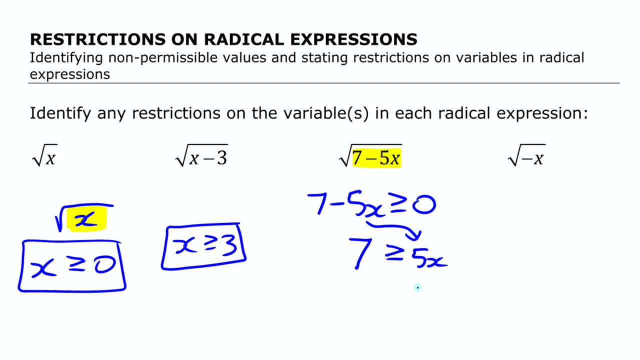 and over here like this: And then if I divide both sides by 5, I get that x is less than or equal to 7 fifths or 1.4 if we're using decimals. That's the restrictions on the variable in that expression. 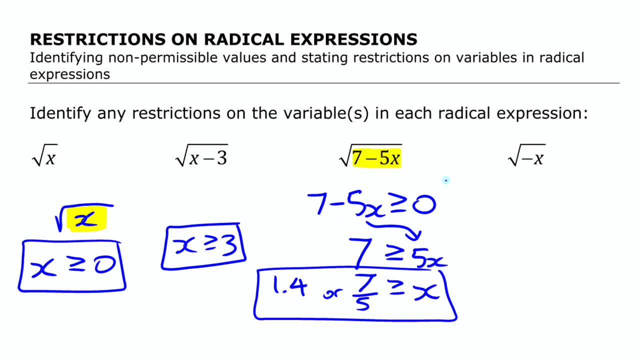 Now, incidentally, if you were solving this by moving the 7 over, let's say you moved the 7 over and you made it minus- 5x is greater than or equal to negative 7 if you moved it over there. If you move that 7 over to the other side. 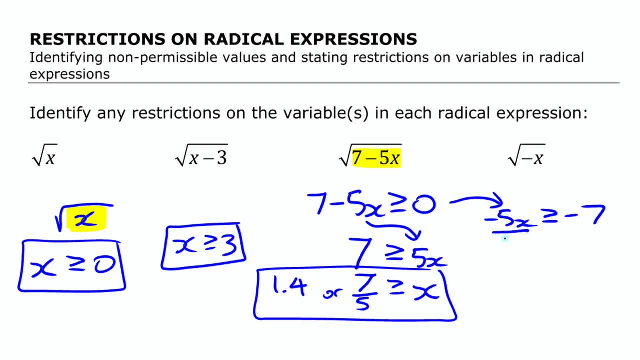 if you have that and you divide both sides by negative 5, this is going to become x over here, This is going to become positive 7 fifths. But since you divided by a negative here, you need to reverse that inequality sign. 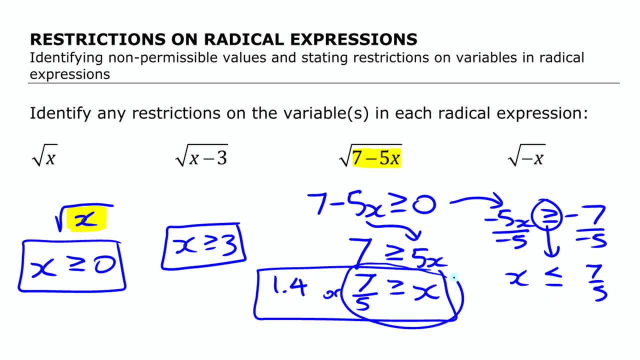 You get the same thing either way here. This says x is less than 7 fifths. This says x is less than 7 fifths. Important to know there. Let's look at that last one Square root of negative x. We can think about this: 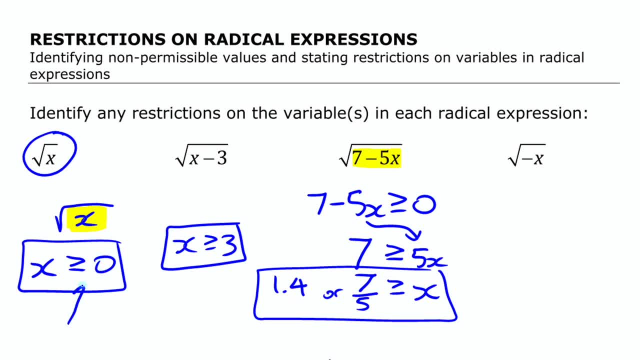 When we had square root of x, the values had to be: x is greater than or equal to 0. If we have square root of negative x now, you don't want to start thinking: well, that's a negative number, It can't be underneath there. 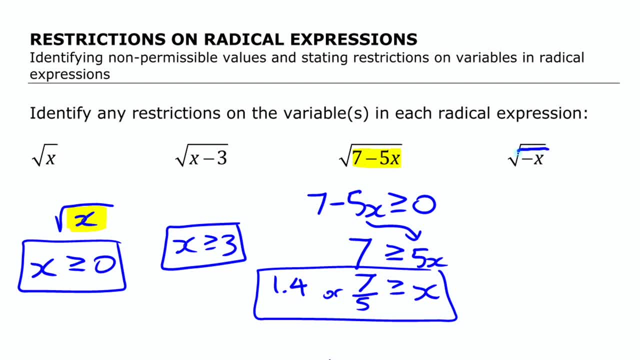 so there are no values that are okay. All this means when you have negative x, you can think about it like negative 1 times x. It just means the opposite of whatever x is. If you have a value like 2, it's just going to be negative 2.. 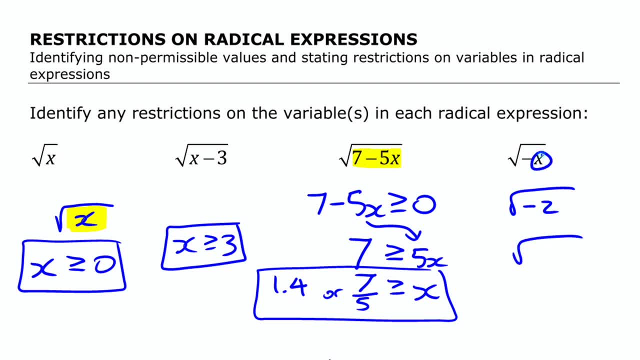 If you have a value like negative 2, it's negative, negative 2.. So it's actually 2.. So the values that are okay in this are the negative values and 0. You can't put positive values in there, because then you'll have a negative result. 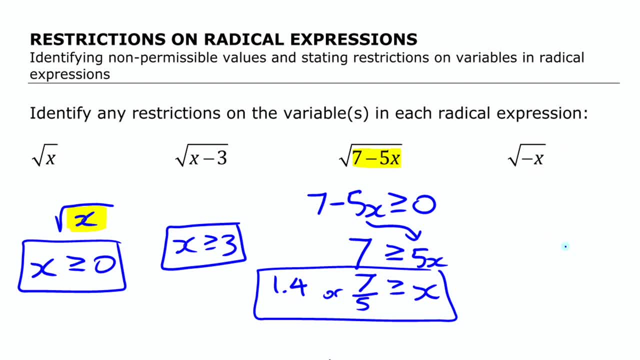 underneath that square root sign. If you can't see that right away, what you can do is say negative x has to be greater than or equal to 0. If you solve this by dividing both sides by negative 1, you get x and you get 0,. 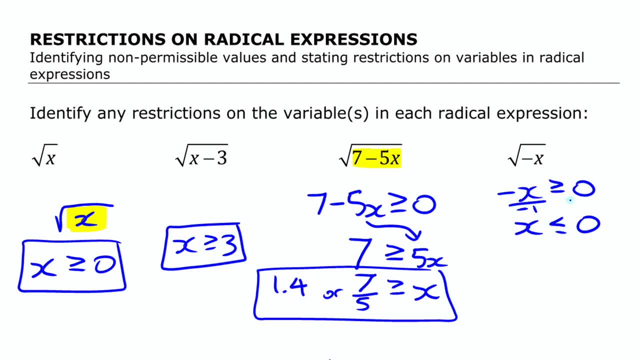 but you have to flip that around because you're dividing by a negative, Divide by a negative. you've got to flip it around. So this one, actually x, has to be less than or equal to 0.. Let's try some more here. 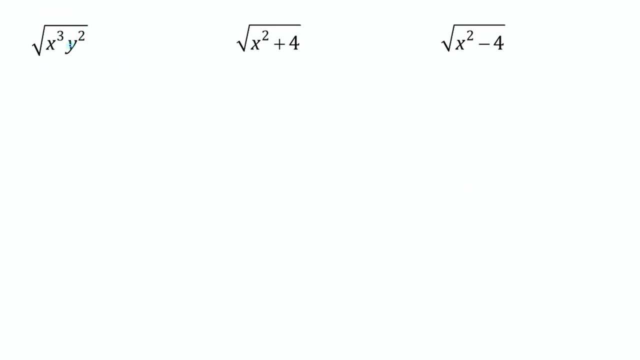 We're going to look at this one. We have two variables And we'll think about the possible values for either variable. Let's start with the y, Because it's squared. you can actually have any possible value underneath there, Because if you have 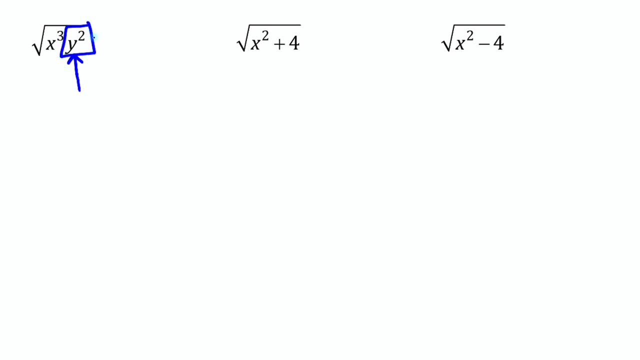 a positive number squared, this will be positive, But also if you have a negative number squared, the result will be positive. A negative number squared is a positive And of course you can have 0.. So the values of y can be any real number there. 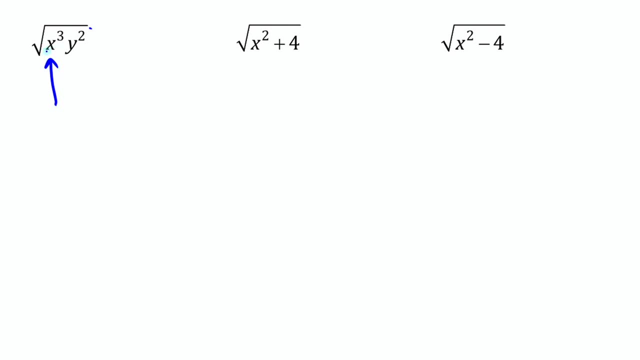 Whereas the values of x here, when you raise something to the third power, if it's a positive number, no problem. 2 to the third is a positive number. Even if you have 0 to the third, it's not a negative number. 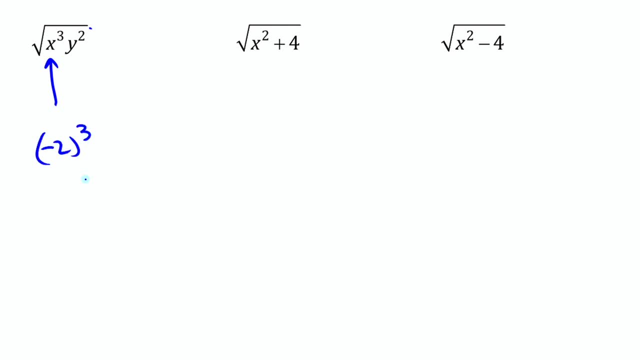 If I have, say, a negative number, like negative 2 to the third, that's negative 8 and that's not okay to have underneath that square root sign. So just the same way as above the values of x here have to be: 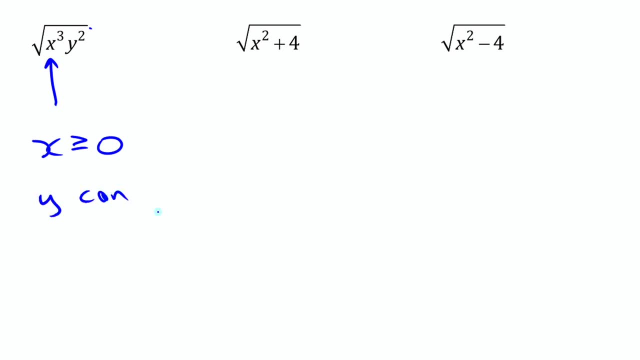 greater than or equal to 0.. But y can be any real number. This next one here: square root of x squared plus 4, for the same reason as the y squared over here, x squared. if you're going to square the value of x, 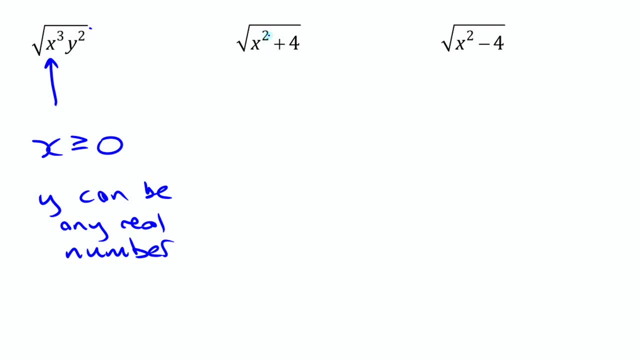 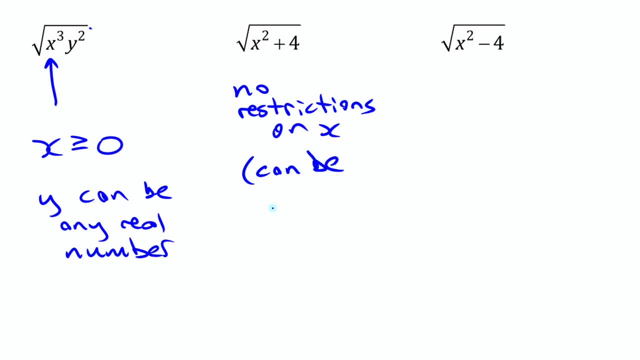 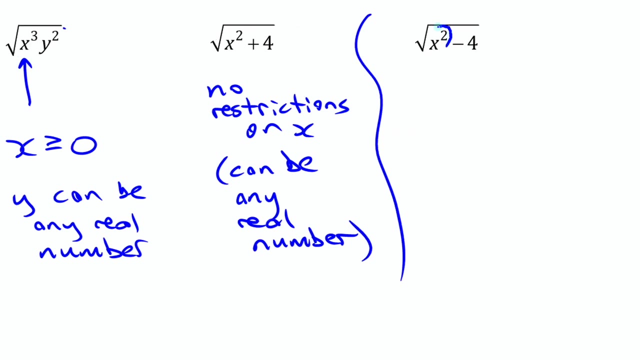 No restrictions on. x can be any real number. This expression looks slightly different here: x squared minus 4.. We need to think about what that means for this. x can be any real number. here This expression will always be a positive or 0.. 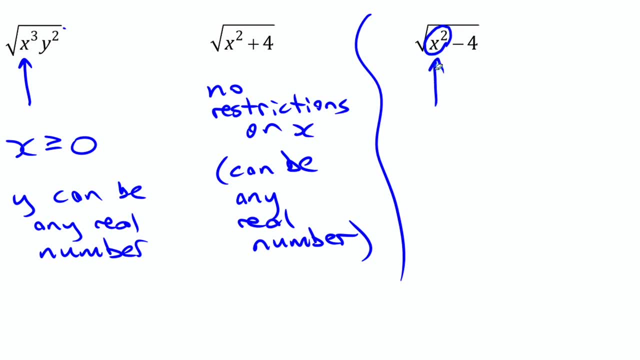 That expression, that x squared will never be negative. So x squared minus 4, we need to think about what that means. We're subtracting 4 from it. So we need to think about what's possible here, Because if you're going to square that and subtract 4, 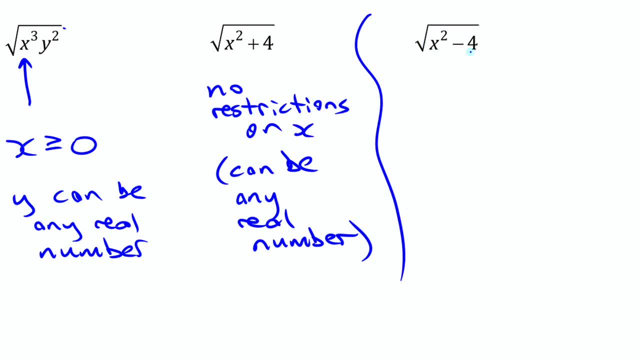 we need this entire thing to be greater than or equal to 0.. So we can think through and say: well, we need this value to be bigger than 4.. x squared has to be bigger than 4.. For x squared to be bigger than 4,. 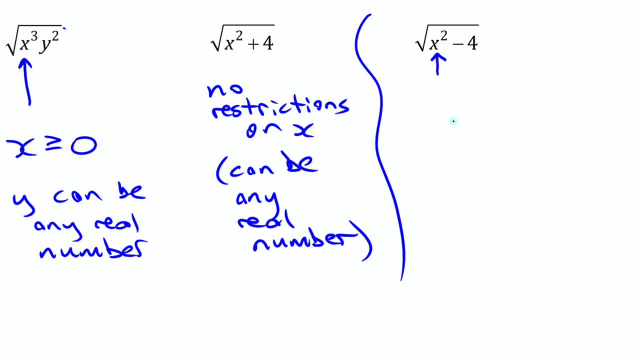 there's actually two possibilities here: x- squared. x squared is going to be bigger than 4, x can be bigger than or equal to 2. if it was 2 or 3 or 4, then this is going to be bigger than this.